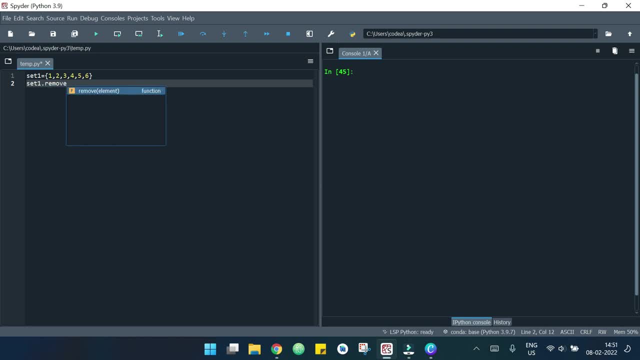 is set, one dot remove and the element I want to delete, that is four. After that I will print my modified set. Now I will hit the Run button and you can see that the four is gone from the set. We also can use the discard method to do that. I will just delete the. 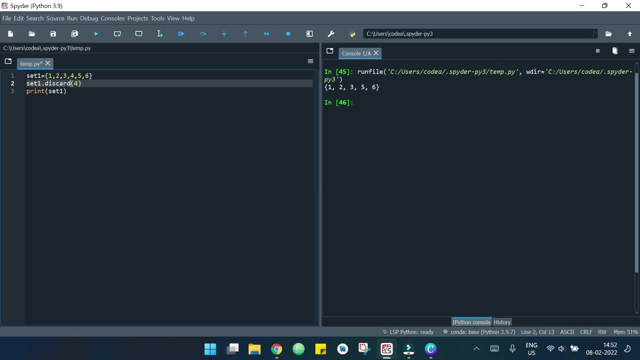 remove and add here Discard. Now, if I run the code, this is the code, This is the same output you can see. okay, Now let's try this with another, another element, suppose one. Now, if I run the code, we can see that the two is not present in the modified. 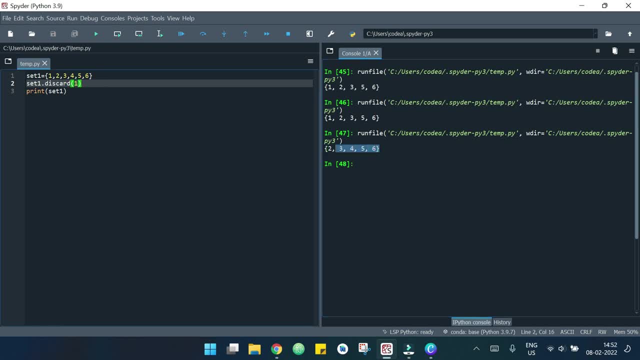 set one. Okay. Now the difference between the remove and discard is when I use the remove method, if the item to remove does not exist, remove will raise an error, But when I am using the discard method, That will not raise an error. now Let's see this with an example. Suppose I am using 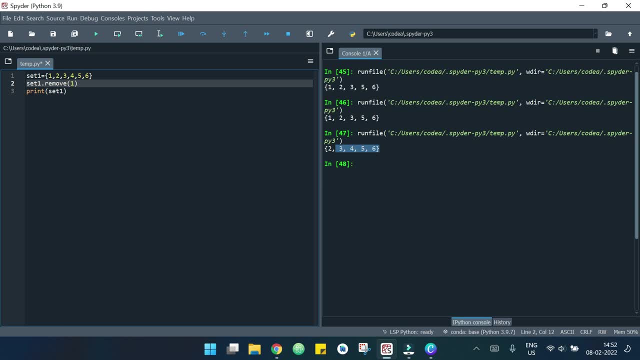 the remove method and I want to delete the five. now we can see that the five is present in my set. Now if I run the code, that operation is successful. but here suppose I write a element that is not. that is not present in my set. suppose I write 10, So if I run the 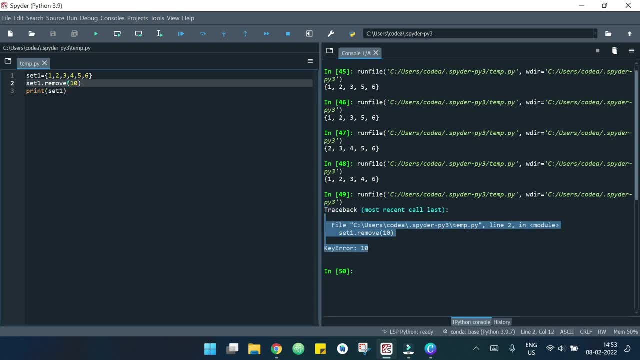 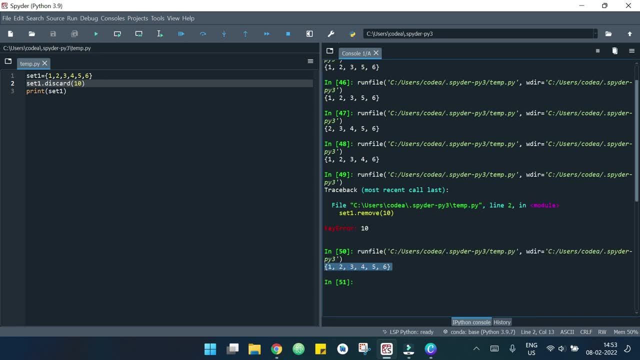 code. But if I do this using the discard method, this will show no error, as you can see here. Okay, now we will this. now we will delete element. Now we will see an example of deleting element using the pop method. pop method always removes. 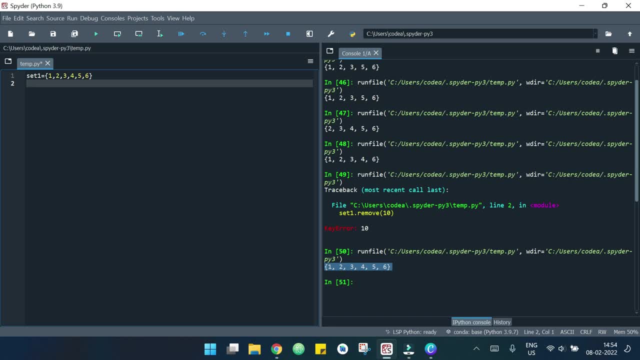 the last item. but in set the items are unordered, So we don't know that which item will be deleted. So let's see that using an example. So to do that, I will write: set one dot pop. Okay, now I want to store the deleted element. 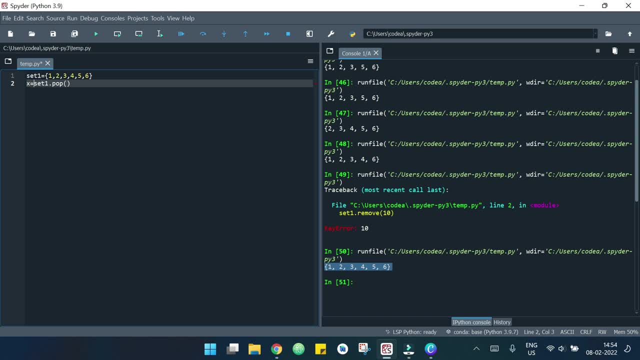 in a variable. So I am declaring a variable x, in which the deleted element will be stored. Now I will print the value of x, because of which we will be able to identify that which element is deleted. Now I will print my modified set, which is set one.